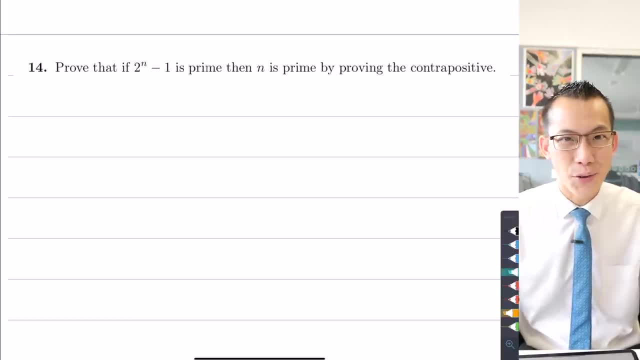 We're going to prove this result about prime numbers and powers of two, And this is a really cute sort of question because the particular content of the question actually has some really interesting historical implications for mathematics and its development over the century. So let's have a look. Prove that if two to the n minus one is prime, then n is prime. 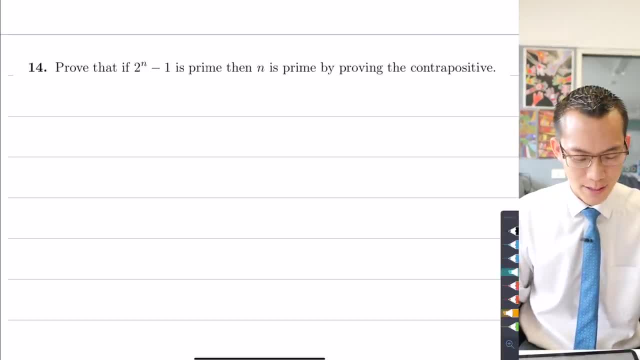 by proving the contrapositive. Okay, let's think about this for a second. For starters, the reason why I said this is a cute question is that two to the n minus one, this is not just some random result. Two to the n minus one. obviously it's an odd number, because two to the n is always. 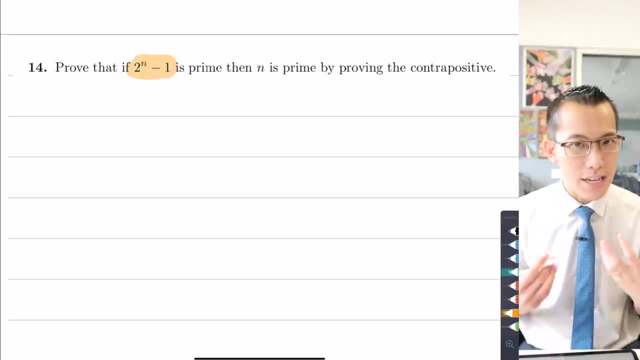 going to be even, But two to the n minus one often is a prime number. It's not just any prime, It's what we call a Mersenne prime, named after a French mathematician who discovered that this was a nice and convenient way to develop or to find prime numbers, particularly very large ones. You 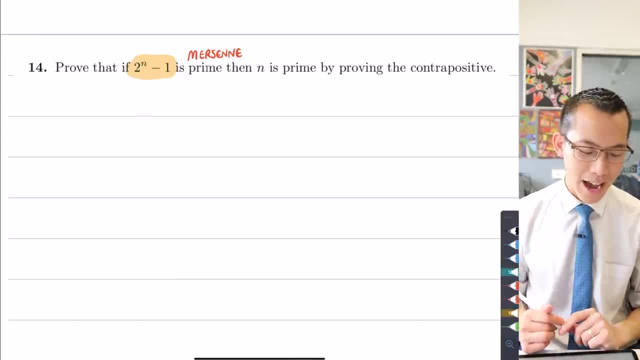 know when things are off the top of your head. you know when things are off the top of your head To an exponential. they grow super fast. In fact, all of the largest prime numbers that we've discovered, you know numbers that go for hundreds and hundreds of digits, that you know supercomputers. 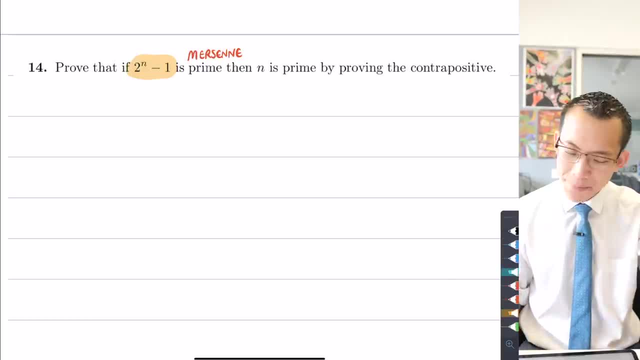 are crunching through and trying to calculate: Is this thing prime? Is it composite or whatever? All of the large primes that we know about, they're all of this form, They are all Mersenne primes. So that's why this is not just you know, something we can prove by the. 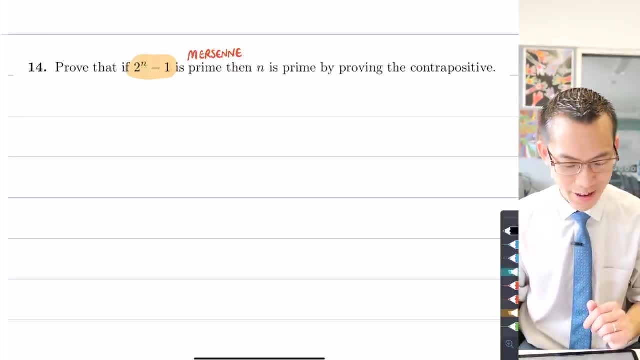 contrapositive, It is also having historical value. How do we prove this? Well, because the question has given us this kind of well, a pretty heavy note. right, Use the contrapositive. What I have to say is, how do I get the contrapositive out of this statement? And then I will try and. 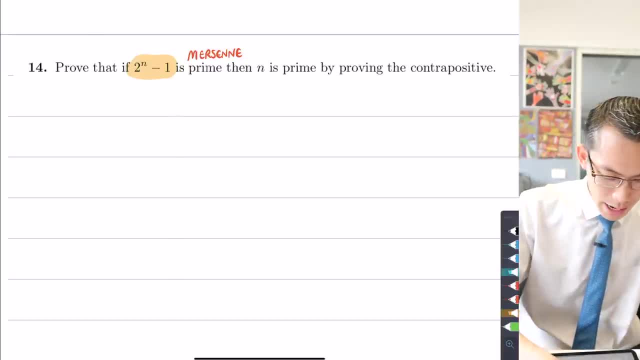 prove that directly. So you can see here: if 2 to the n minus 1 is prime, So 2 to the n minus 1 is prime, is the first half. It's the antecedent clause or statement within this implication. 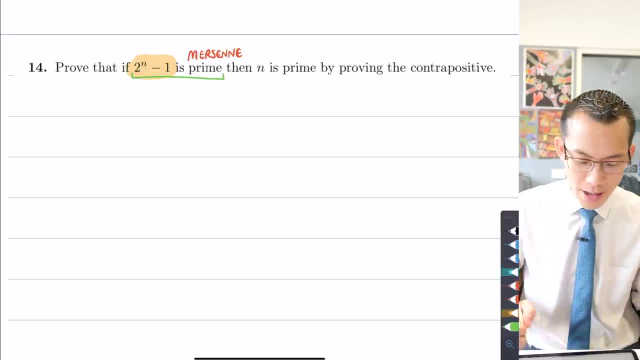 I'm going to negate that and put it rather than at the beginning, I'm going to put the end And then you've got this second half, the consequent statement. Then n is prime. So I'm going to negate that as well and put it at the beginning. So how do I? 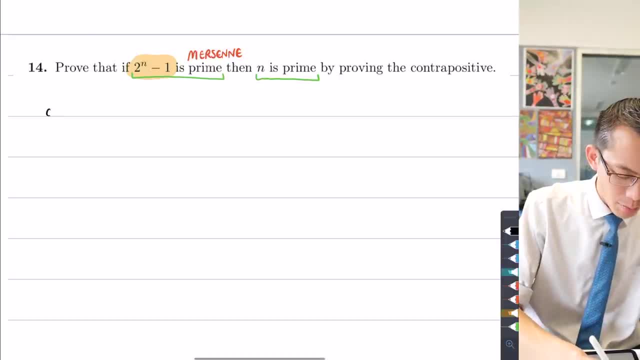 state that I can say this is the contrapositive. so I'm just going to write that here. The contrapositive- not q implies not p in this particular question- is: if n is not prime- just very simply negating it- then 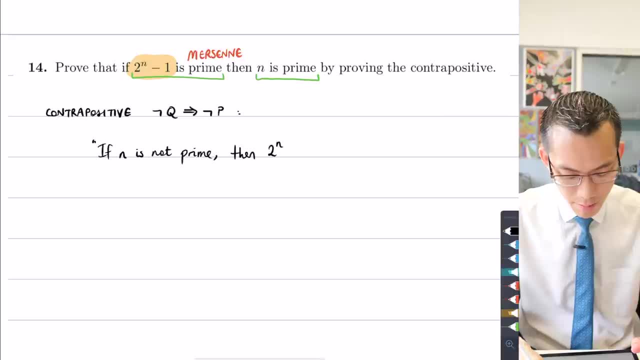 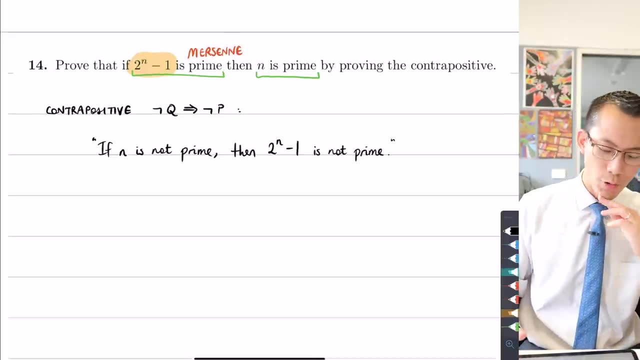 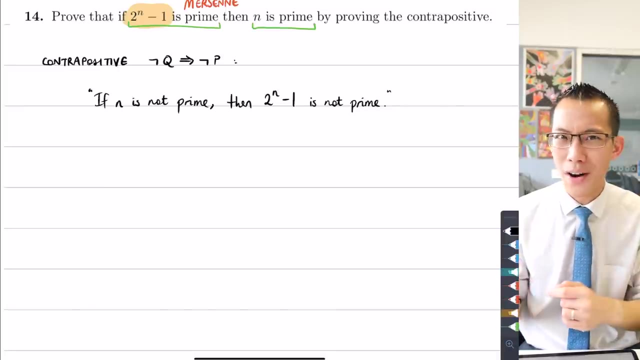 here comes not p, then 2 to the n minus 1 is not prime. Now I did slip in a little bit before. You might want to say the word composite here. right, But we do know there are numbers that are neither prime nor composite, Numbers like 1, 0,. 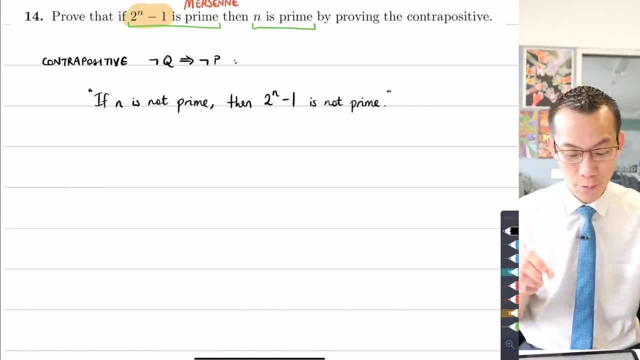 weirdos like that. They are, of course, very important numbers for not sitting in these categories, But that's why I can't say if n is composite, then 2 to the n minus 1 is composite. That's not the full negation. I need the exact. 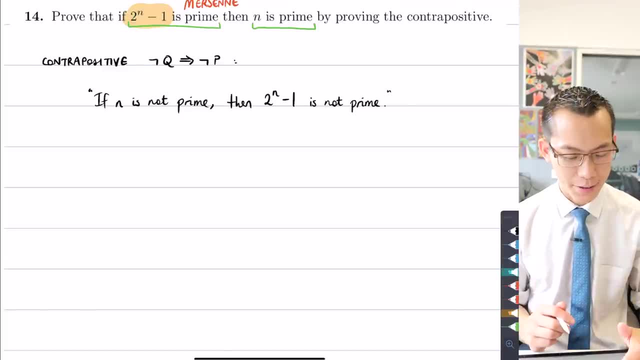 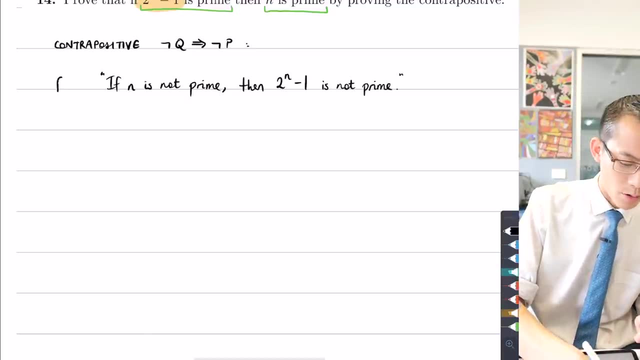 opposite of the statement that we began with. statements, in fact. How do we go about this? Well, I want to think about: if n is not prime, what can I like? This is what I'm required to prove. What can I say about it? Well, it's to do with factorization. 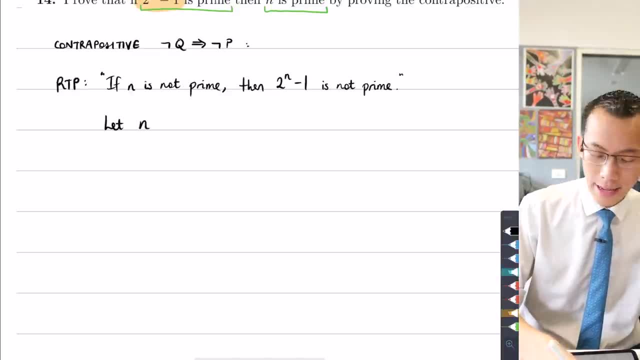 right. So what I can say is: let this number n, let it be factorized into. I mean, who knows how many factors it has, but it's going to have at least two that are not going to be 1.. So I can say: 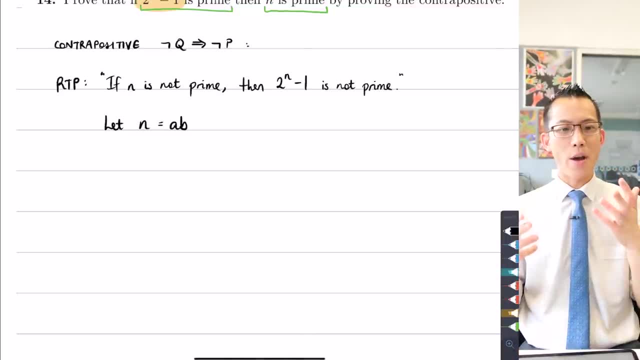 say n equals say a times b, where a and b, they both need to be whole numbers. a and b are whole numbers and of course if a or b were 1, then that would be a problem, right. 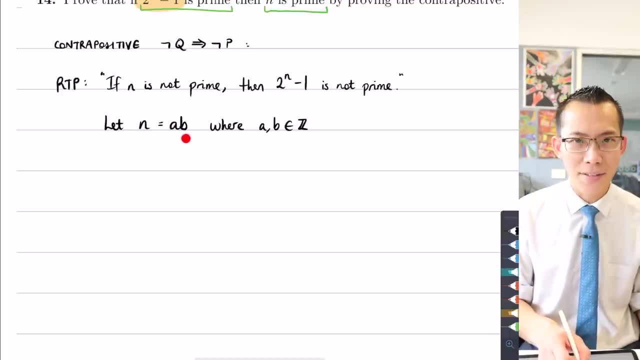 Because then I could say, oh, what if n was 1 times 11? Does that count? And the answer is no, of course. 1 times 11 is 11, 11 is prime. so I have to say I have to restrict. 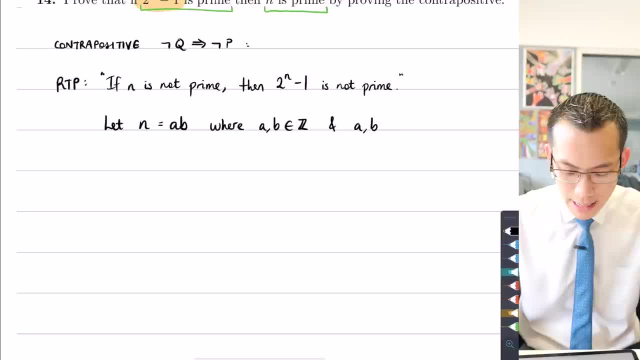 even further, and a and b cannot equal 1.. So here's my groundwork. What can I do with this? Well, I want to prove that if n is not prime, if n can be written like this, then 2 to the n minus 1 is also not prime. So in other words, I can say 2 to the power. 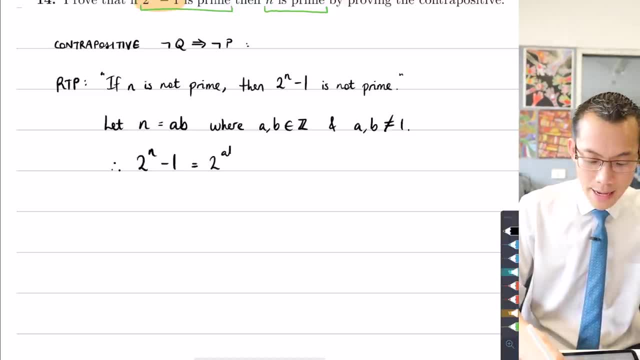 of n minus 1 equals 2 to the power of a, b minus 1.. Hmm, Then you might think: oh, I am stuck because there's not much that it looks like you can do with this thing. I want to prove that this thing is not prime, but it doesn't look like there's any obvious manipulation. 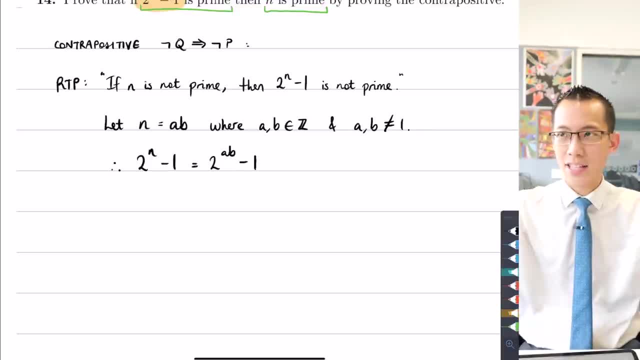 you could do to it. If you were being asked to simplify and you had some expression or some function, and this was the last line that you ended up with, I think most of us would say: I'm pretty happy with that. It is as simple as it gets. So where do I go? 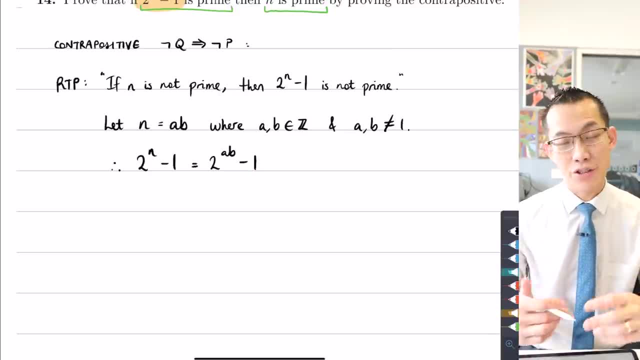 next, There are no obvious steps. Well, it is kind of true that this is as simple as it gets. We need to complicate this. I'm going to be able to write what's going on here. I want you to remember. let me use. 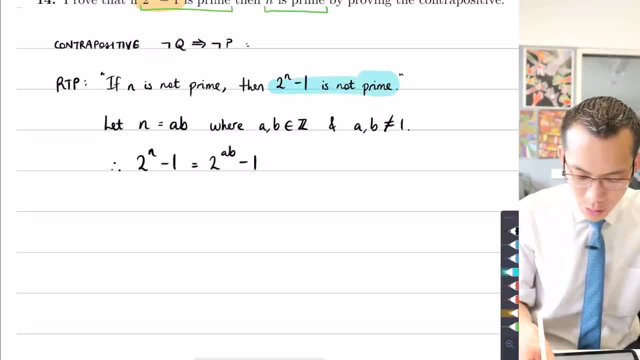 this highlighter that what does it mean for 2 to the n minus 1 to not be prime? Well, it's very similar to n not being prime. I need to be able to write some kind of factorization. I need to be able to say that this, this term here, or expression, rather, I should be able. 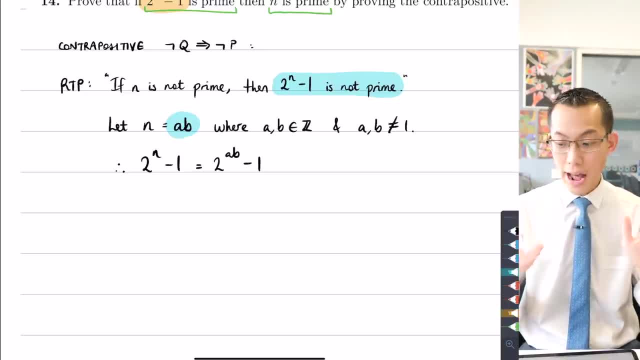 to write it as something times something else where neither of those things is 1.. If neither of them are 1, then I'm going to be able to write something times something else where, and their whole numbers. then well, there's a factorization, so it's not. 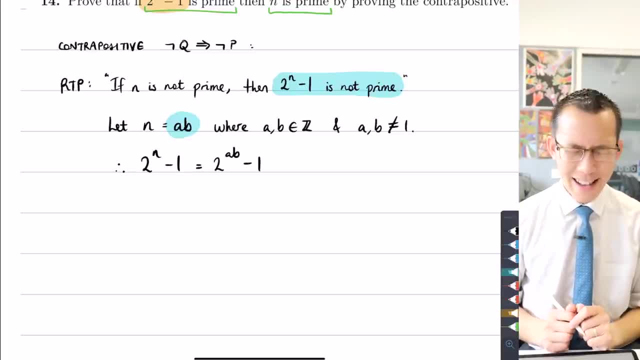 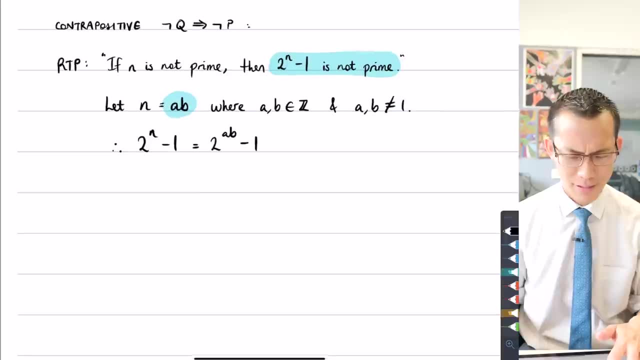 going to be prime, so that's where I need to head to. How can I factorize this thing? How can I work with this term here and come up with something factorizable? Is that a word, Composite, I guess, To show that this is a factorizable object I want. 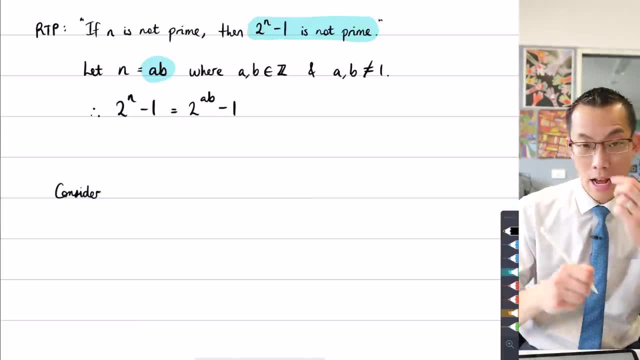 to think: well, what objects vaguely look like this, that I do know how to factorize. Now you can see from the start: here you've got this term, here it's got an index, it's got the whole thing is a power. and then you take away. 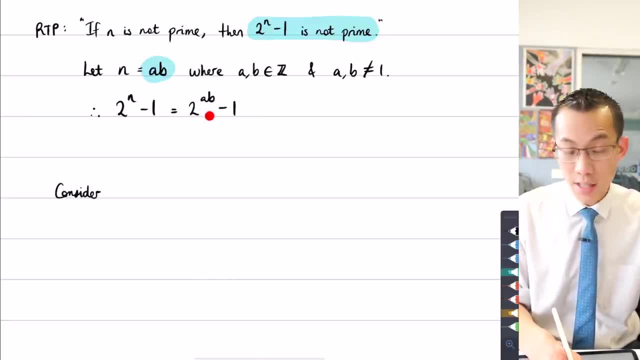 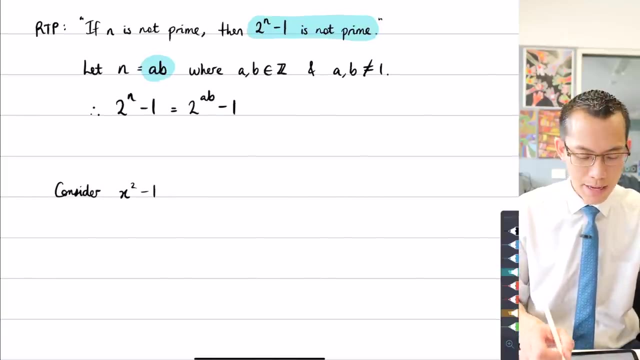 one. I actually do know how to factorize a bunch of things that are somewhat in that format. Something raised to a power minus one, The simplest one that we know about. we learnt about years ago. we would call that the difference of squares, but this is a particular difference of squares, not just a squared minus b. 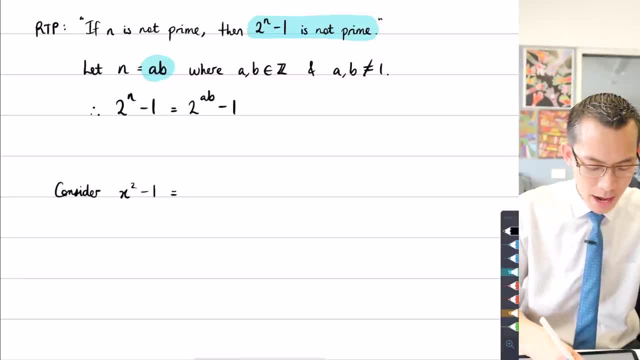 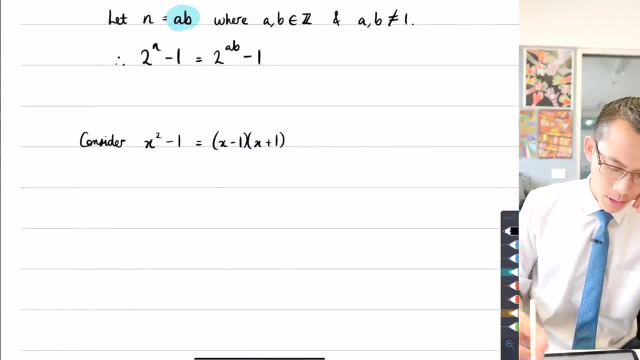 squared, but take away one. this is really easy to factorize. in fact, it's just x minus 1, x plus 1. that's great. Now, the only problem with using this result is that it relies on the fact that the index here is two, and I don't know what this index is. it's not going to be two, it's going to be. 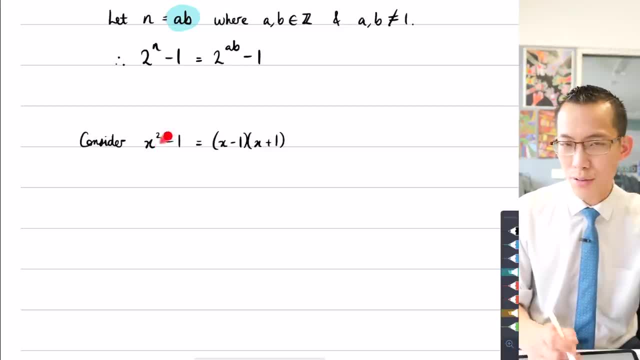 some non prime number. so I need to go from this to something something larger and more complicated. So let's see if we can establish a pattern of factorization that can help us, following this pattern, to work with this object up here. Let's consider a higher power, because I'm going in the direction of 2 to the power. 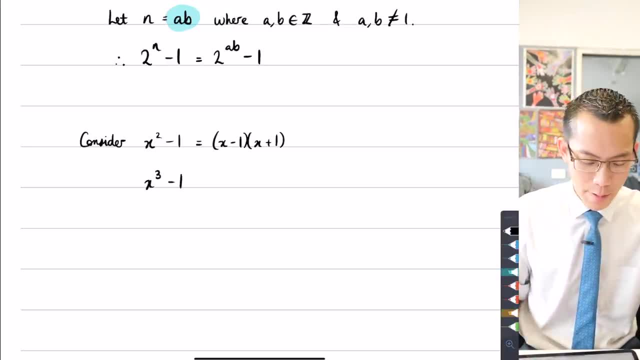 of a, b and a b, I know, as a non prime number, is going to have to be a bit bigger than this. What's the factorization of x cubed minus 1? Now you might know this one. this is a difference of cubed. it's actually remarkably similar to the factorization. 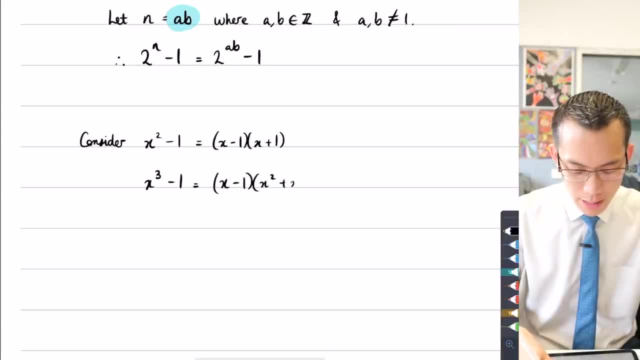 for difference of squares it's x minus 1 and then x squared plus x plus 1.. You could expand this out to contain yourself if you haven't seen this result before. If you just multiply and distribute through everything by x, you'd get x cubed plus x squared plus x. X cubed plus x squared plus x. I might as well write that down. 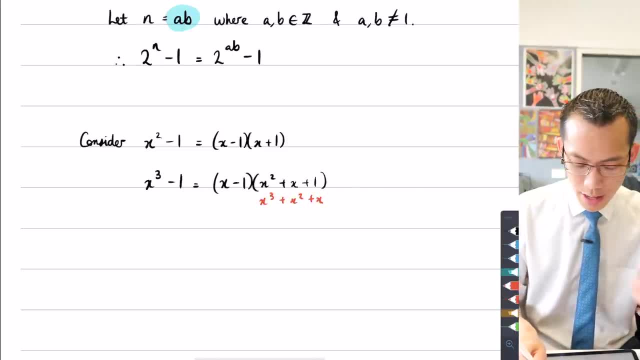 X cubed plus x squared, plus x squared, squared plus X, and then when you distribute the minus one, you're going to get minus X squared, minus X minus one, so you can see the X squared cancel, the X's cancel, and that just leaves you with the X cubed and the minus one, just like you. 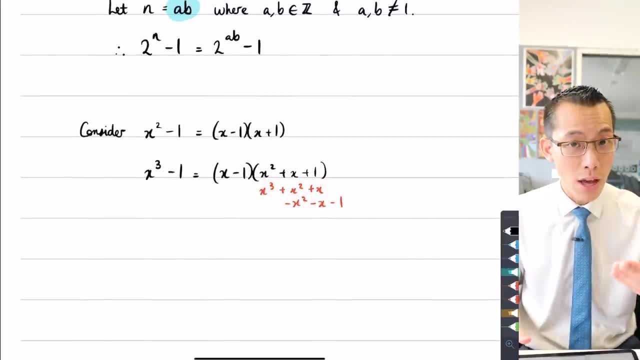 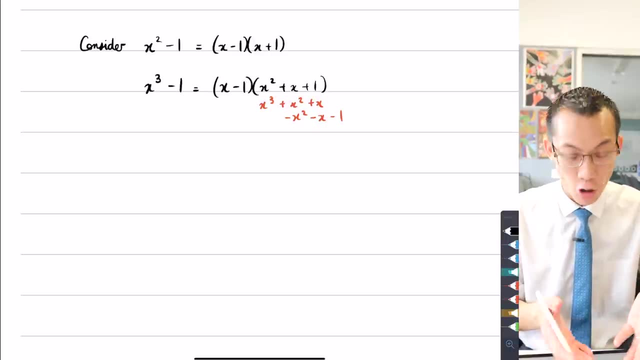 wanted. so this is actually really neat and you can continue this pattern. it's actually something which is very useful when you're deriving the power rule for differentiating X to the power of n. that's the objects that I've got here. right, I can say X to the 4 minus 1. I just want to establish the pattern here. 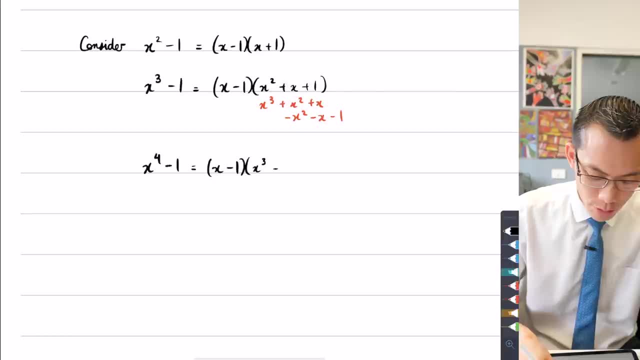 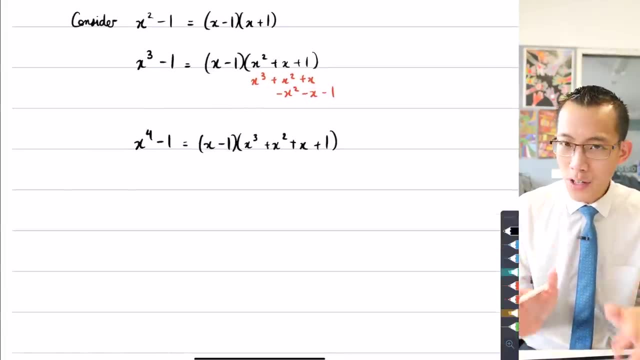 it's going to start with an X minus one and then it's going to go X cubed, X squared, all of the X terms all the way down to 1. so I want to try and get to something like this. this a beat right. well, if I go up to say, and you'll see, 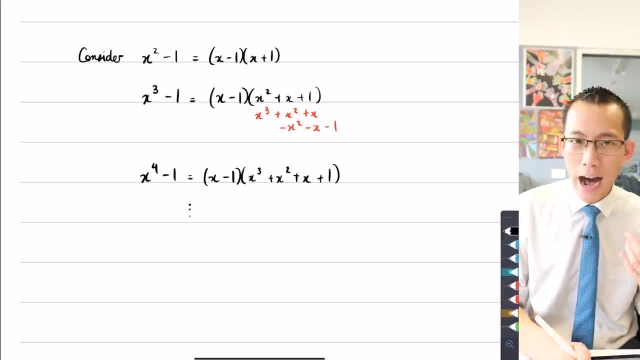 why I'm choosing this in a second. if I go up to some arbitrary positive integer like B, right, I'm gonna go X to the minus AB, right. so if I go up to some arbitrary positive integer like B, I'm gonna go X to the minus. 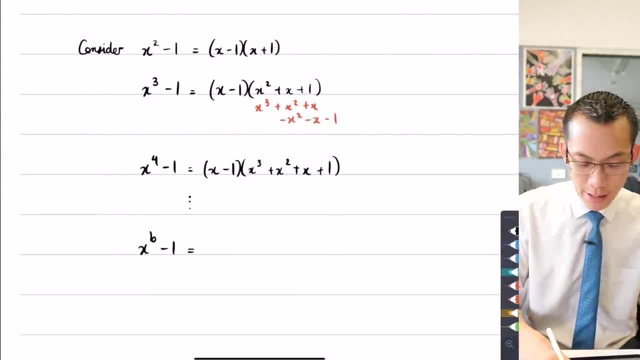 x to the b minus 1 equals, right. how does it begin? well, continuing the pattern, they all begin with x minus 1, right? so you're going to have the x minus 1 out the front, and then what you get is this: uh, it's this long polynomial that has 1 and x and x squared all the way up to, uh, this largest power. 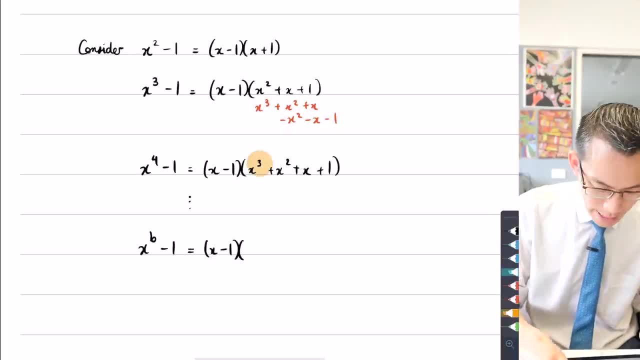 where that largest power is always. just look at it carefully: one less whoa. that was much bigger than i anticipated. uh, one less than the power that you started with. you can see i've got two where i had three and then, even though it's not written there, you can see there's a one hiding here. 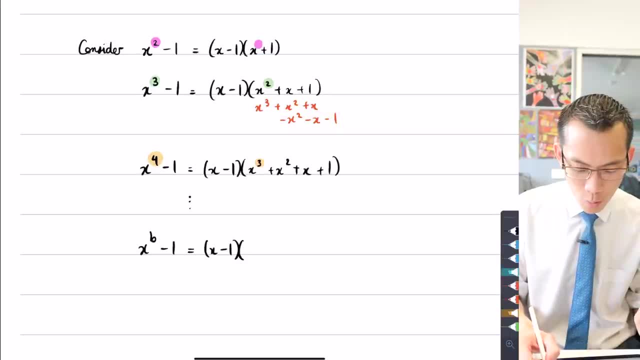 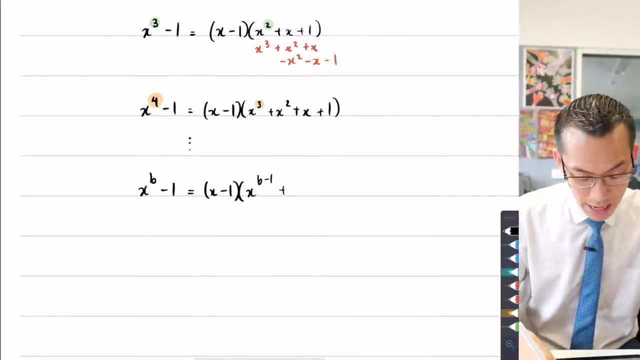 and there's a two. so you can see, i'm going to go from 1 to x, to x squared, and i'm going to terminate on the power of x. just one less than what's in my original expression. so what's one less than b? it's b minus 1. so i'm going to go b minus 1 and then i'm going to have one less than that which. 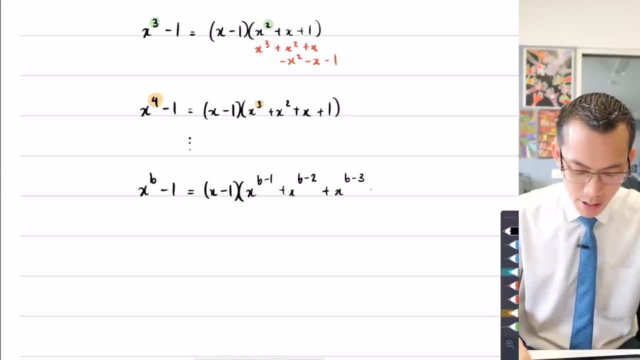 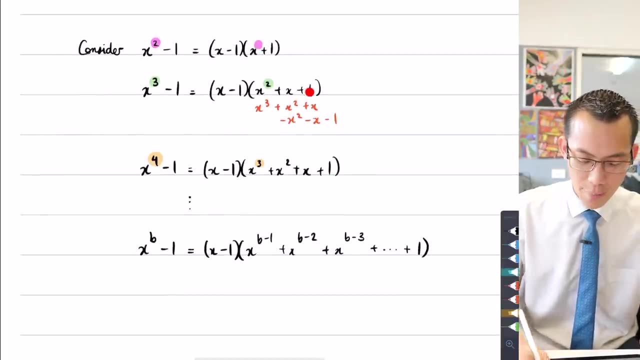 i guess would be b minus 2, continue the pattern b minus 3, and it keeps going until you finish on 1, 1, 2, and 3, which you can see in all of these uh factorizations up above here. now, how does this? 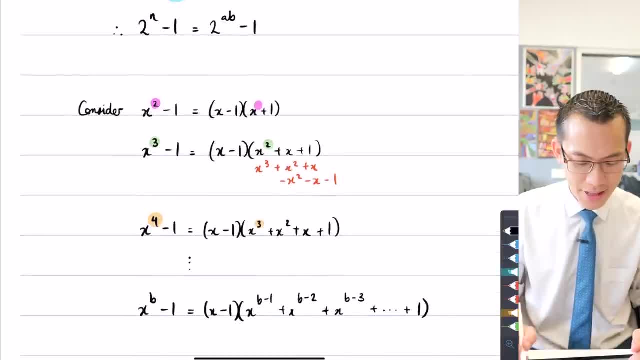 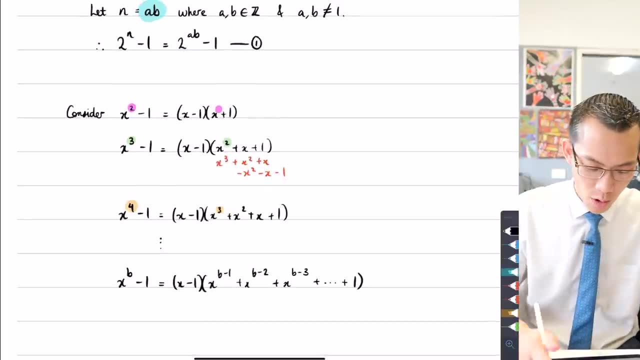 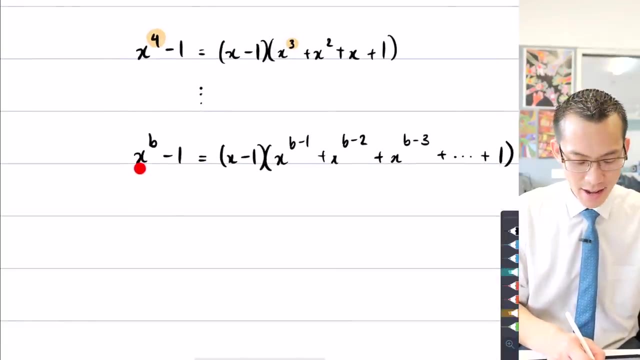 help me. well, uh, think about this right, think about how this is related to this object that we have up here and i'm going to name this. i'm going to call this equation 1 so that i can work with it. i can say: well, if i substitute instead of x, if i put in 2 to the power of a in there, then what i'm 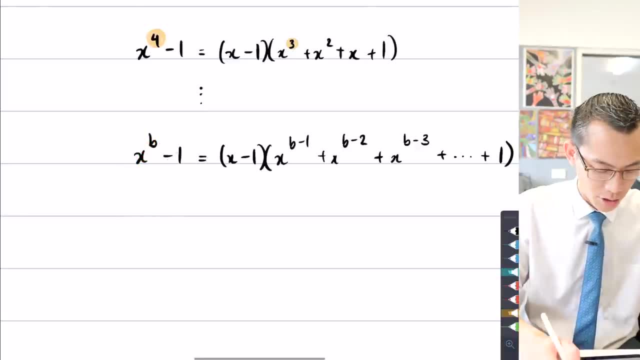 going to have here on the left hand side is 2 to the power of ab, so i'm just going to go ahead and write 2 to the power of a, that's my chosen. x to the power of b minus 1 equals all right everywhere. 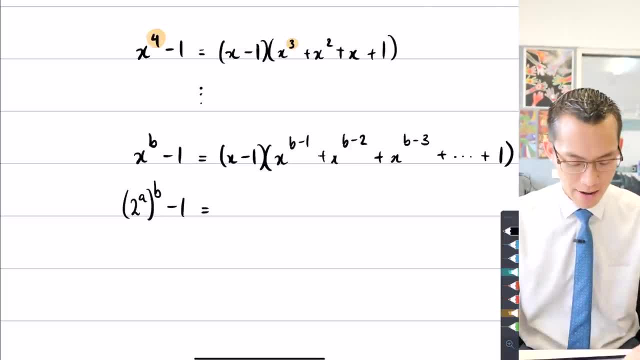 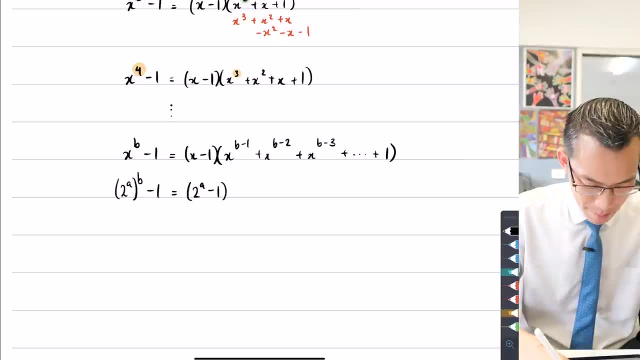 that i had x. i'm just going to substitute it for 2 to the power of a. so let's have a go 2 to the power of a minus 1, and then what have i got here? all right, maybe i'll draw a bigger bracket, so i. 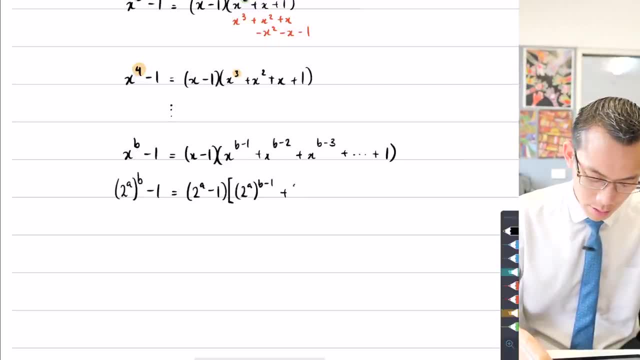 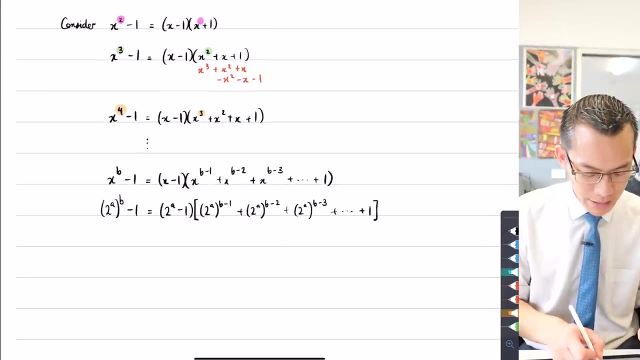 can fit in my 2 to the power of a, to the b minus 1, to the power of a, again to the b minus 2, one more time to complete the pattern b minus 3, and then dot, dot, dot all the way to one. all right, so what have i got here? well, on my left hand side, 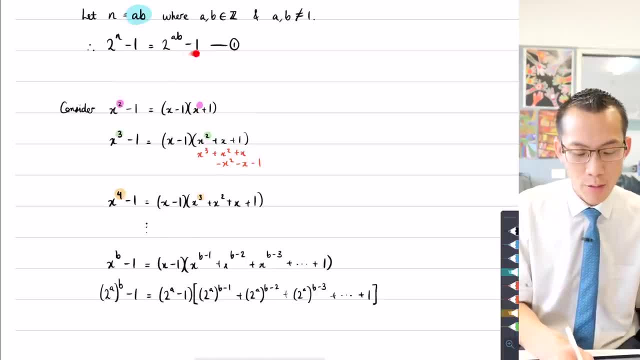 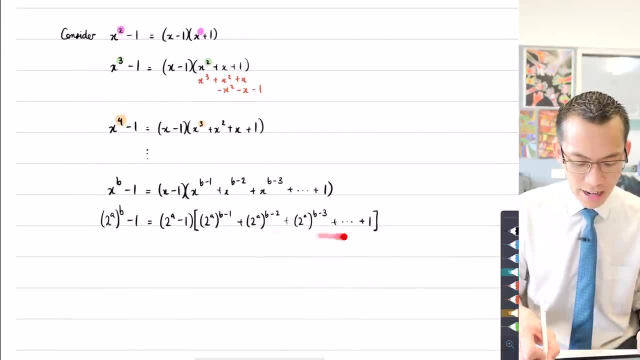 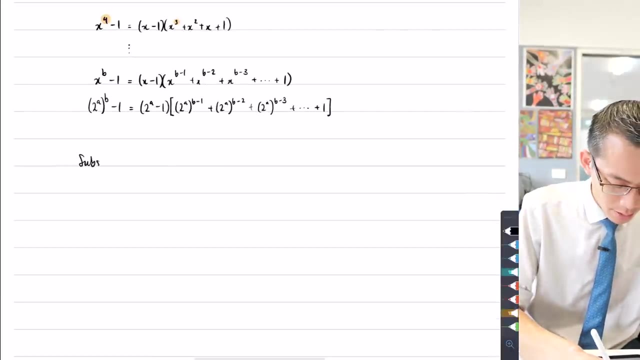 this is where i left off in equation one, right. this was that object where i was like i don't know what to do with this thing. well, now i do know what to do with this thing. i can say: well, i've got this factorization written here on the right hand side, so i can say, uh, substitute this result into one. 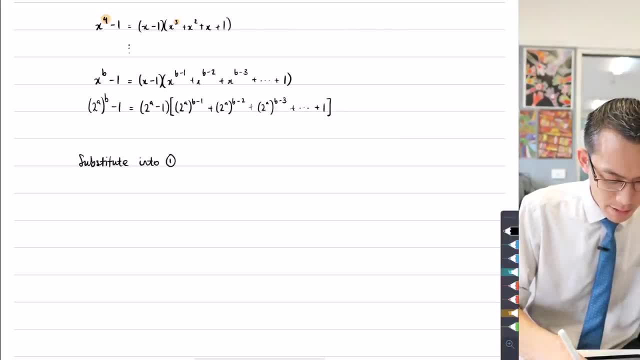 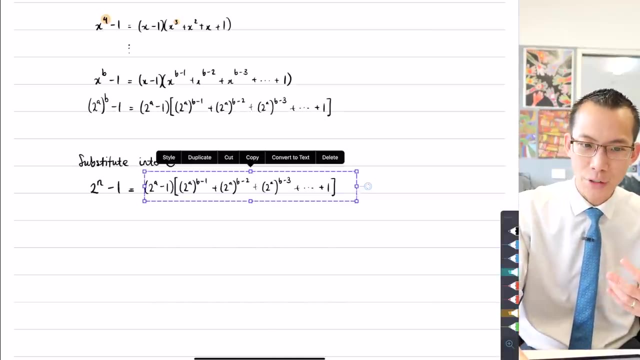 uh, two to the n minus 1, instead of writing it as 2 to the a b minus 1. i'm going to take everything here and duplicate that down. so where does this leave me? i mean, it's a factorization, but we already established that just because you have something times something, that doesn't mean that you're 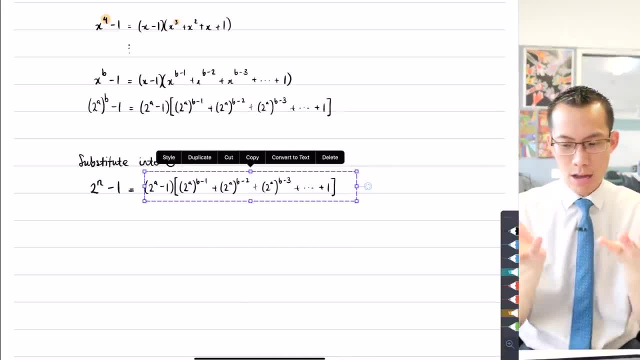 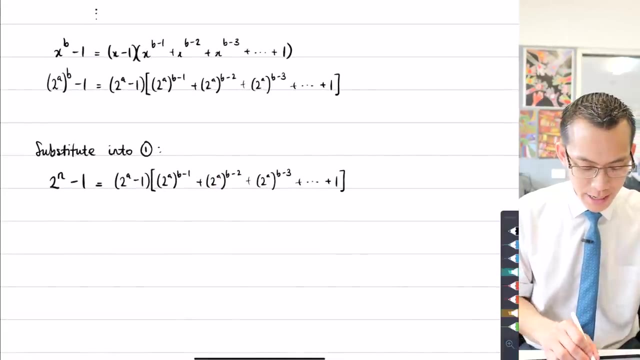 going to have a non-prime number. one of those two factors might be one. so 1 times 11 doesn't mean that 11 is non-prime. so i need to show that neither of these two things- this object and this object- can be equal to one. how do i do that? well, for starters, um, you can see, let's deal with this one. 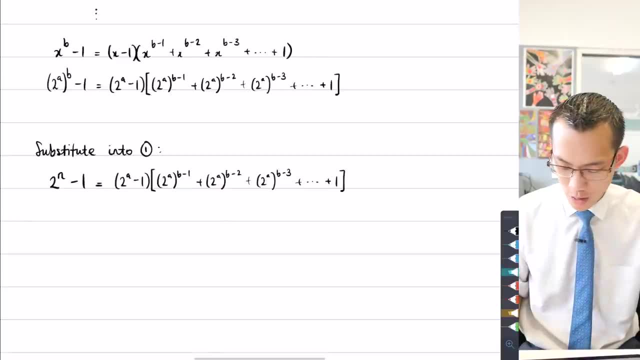 over here on the right hand side. this can't possibly equal to one, because you can see there's a one right there, and then you're adding things to it. right, all of these things that are added to one mean you're going to be bigger than one. so i can say, uh, let's, i'll just leave those arrows there. 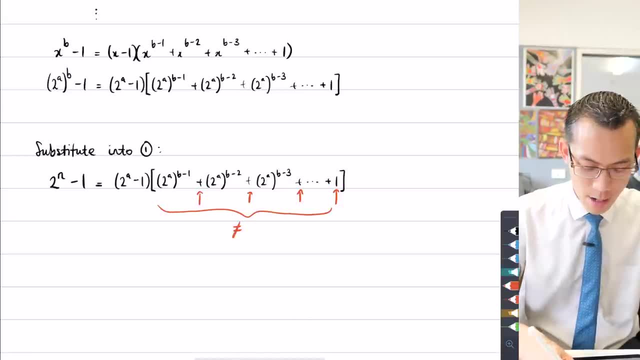 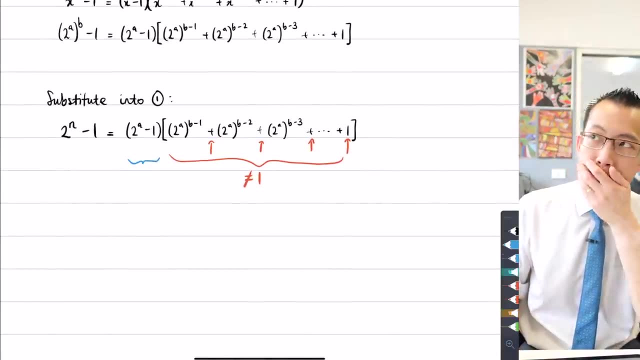 that's fine, everything in here that can't equal one. well, that leaves me with this object on the left-hand side. think about this: 2 to the a minus 1, it can equal 1 under certain circumstances, but we actually know that that's not the case, because of a restriction that we placed on a. 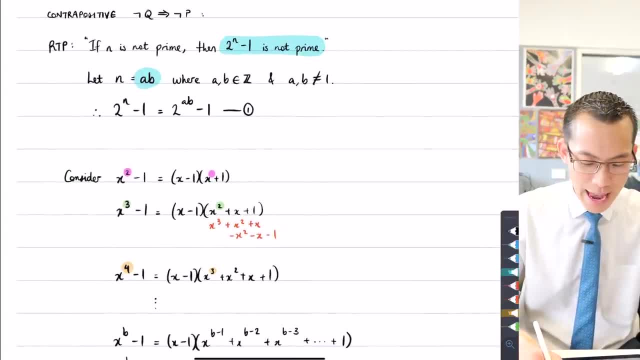 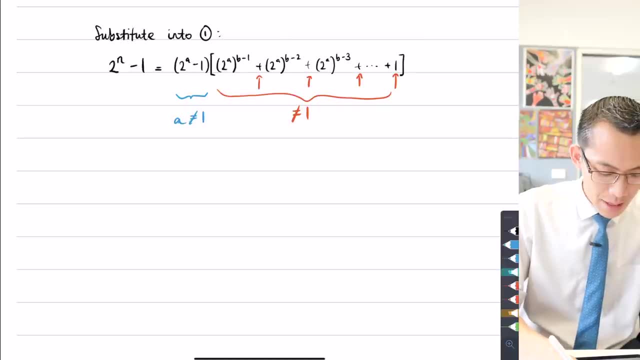 right at the very beginning. You can see over here a and b, they can't be 1, right? So therefore I can say if a can't be 1, then 2 to the power of a can't possibly be 2 to the power of 1,. 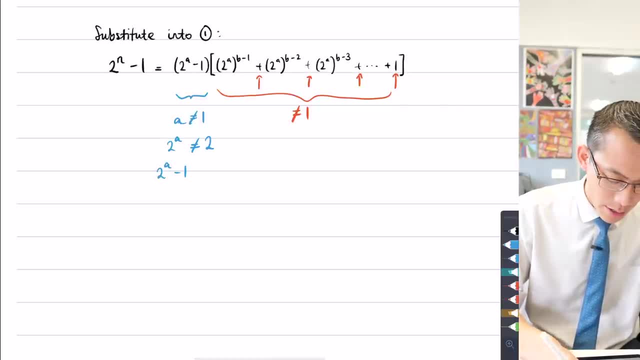 which is 2, and that means 2 to the a minus 1,. that can't possibly be 2 minus 1,, which is 1.. So you can see, I've just raised it to the power of the previous line and then I've subtracted.